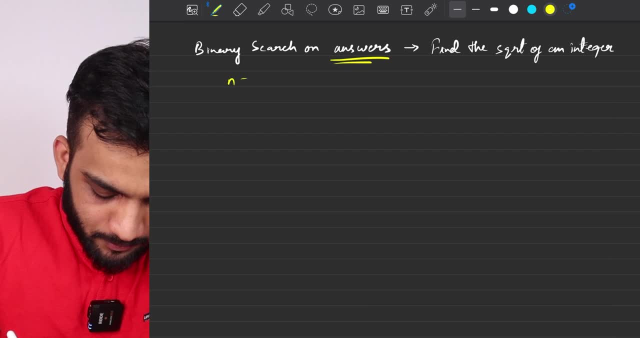 way, The linear search way, imagine I give you n is 25.. The linear search will be: I'll take 1, I'll do 1 into 1, that's 1, that's not 25.. I take 2, 2 into 2, that's 4, that's not 25.. 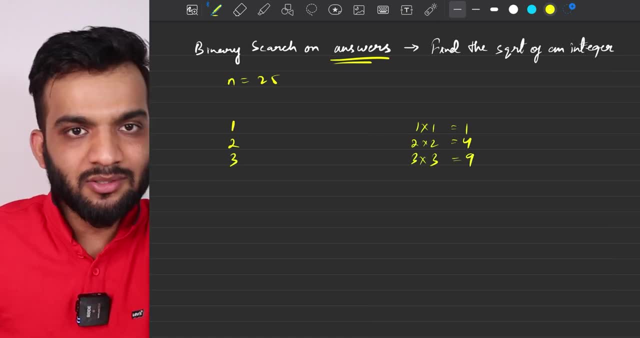 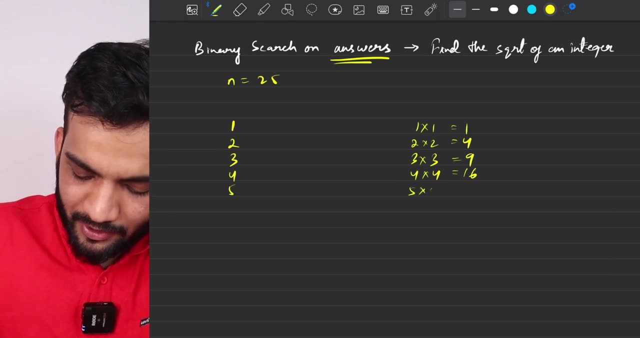 I take 3, 3 into 3,, that's 9,, that's not 25.. I take 4, 4 into 4,- 16,, that's not 25.. I take 5, 5 into 5,, that's 25, and I say, yes, this can be a possible answer. 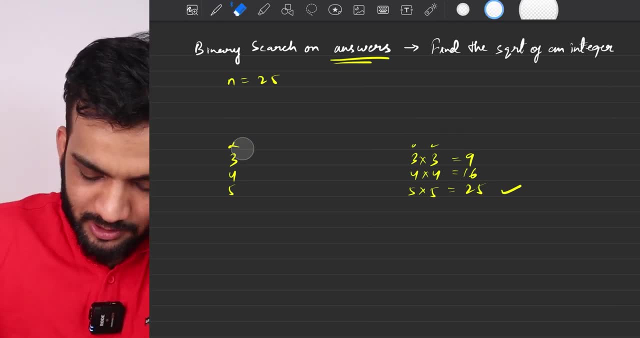 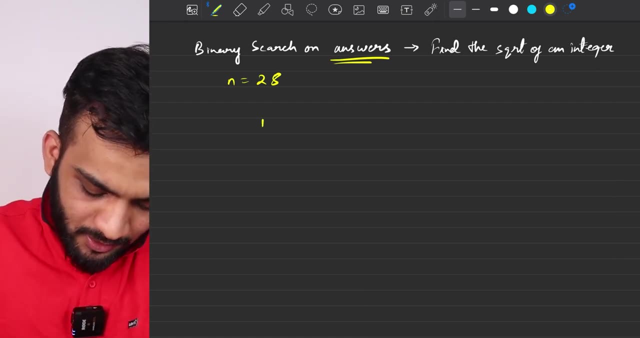 Or what if it was something like: just imagine, instead of a complete value, it was something like 28.. In that case, you'd have gone with 1,, 2,, 3,, 4,, 5, and whenever you had 6,, 6 into 6 would. 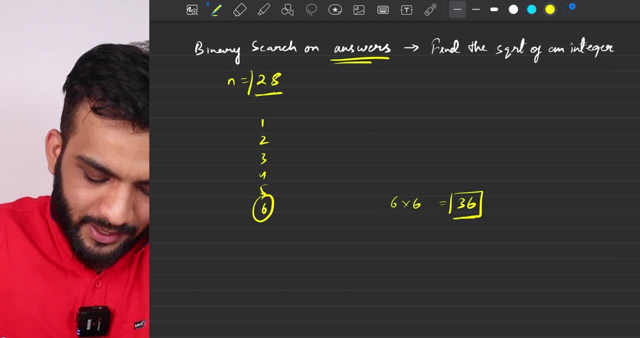 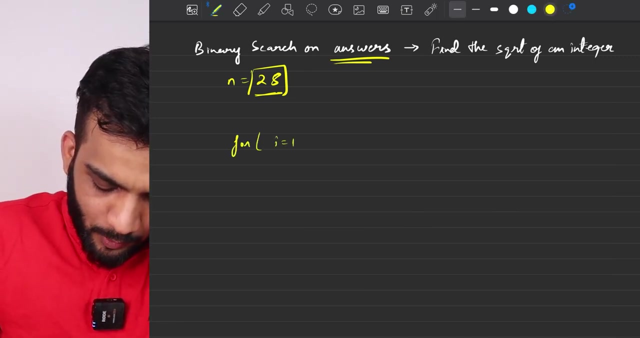 have been 36, and the value 36 would have exceeded 28.. So the possible answer would be: would have been 5.. So we can linearly traverse, right. So what's the code for this? If I have to write the code, can I say the code will be for: i equal to 1, i lesser than maybe we can just. 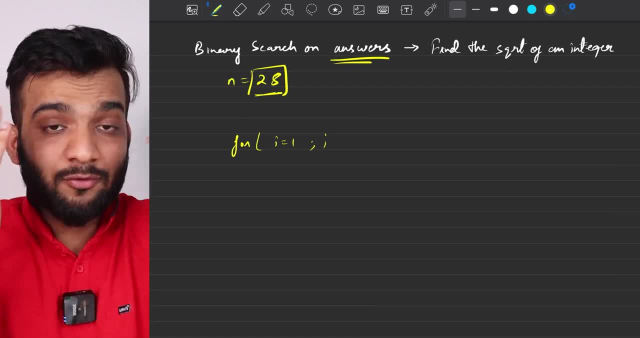 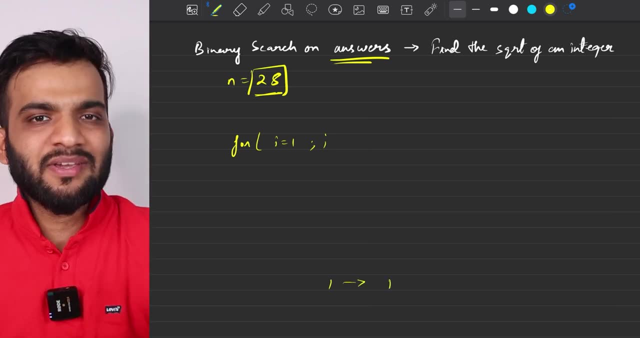 leave this. What can be the maximum answer? if I have to ask you For any value, what can be the maximum answer For 1, it's 1 itself. The number itself can be the maximum possible answer and it will not be. But if I have to write the code, what can be the maximum answer For 1, it's 1 itself. 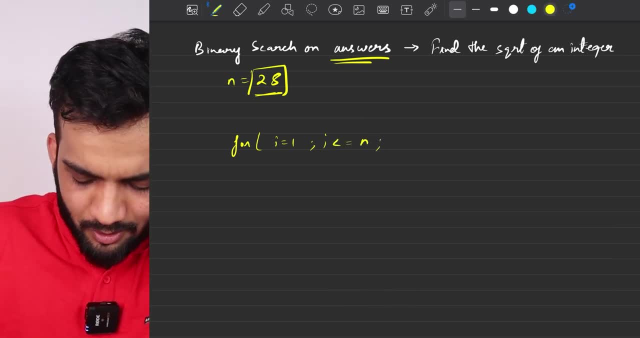 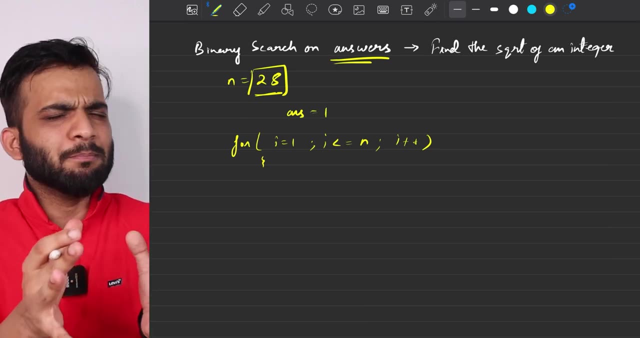 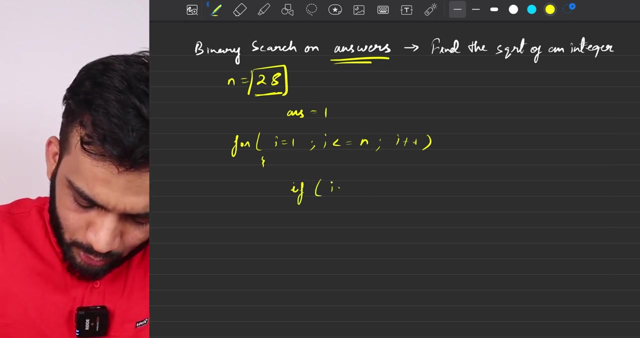 But the maximum I can go as still n. Obviously we will stop way before that, but we can go till here. Now maybe I can keep the answer as 1, because that's the minimum possible answer as well. So I'll keep the answer as 1, and I'll say: hey, if i into i is lesser than equal to n, then 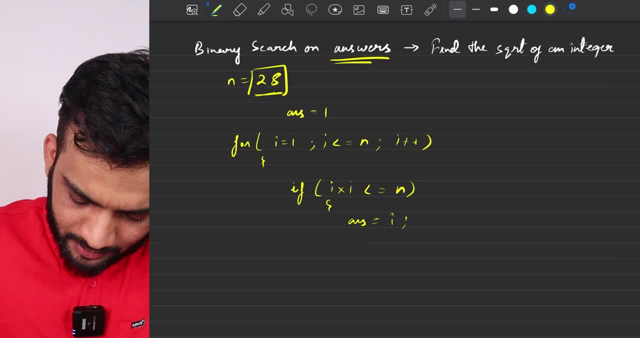 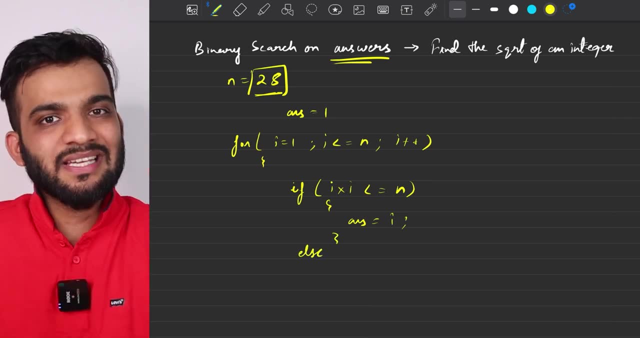 say answer equal to i and continue, Or else, if I'm going to the else part, what does it mean? It means it's greater than n. So I'll say break. Can I do this? I can, So this will be working. 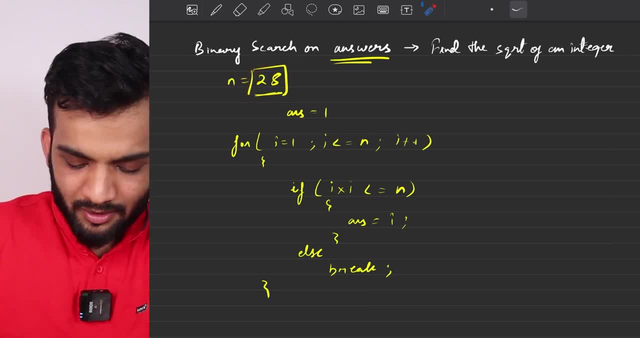 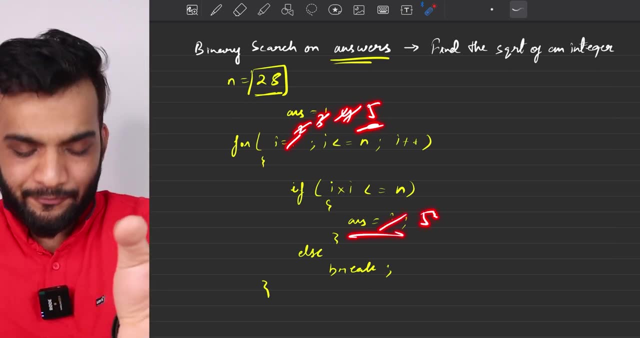 right. So if you take this particular example 28,, it goes for 1,, 2,, 3,, 4,, 5, and the last value answer will be storing is 5.. And after that, whenever i becomes 6,, this condition is false. 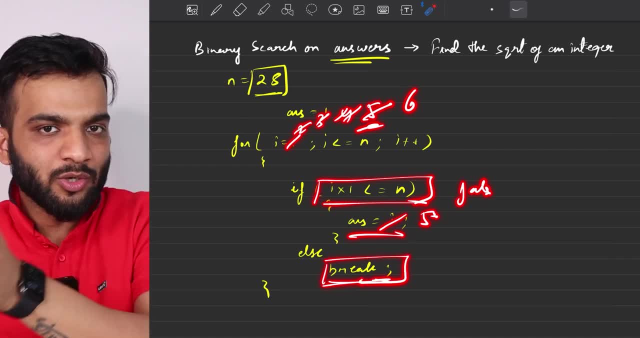 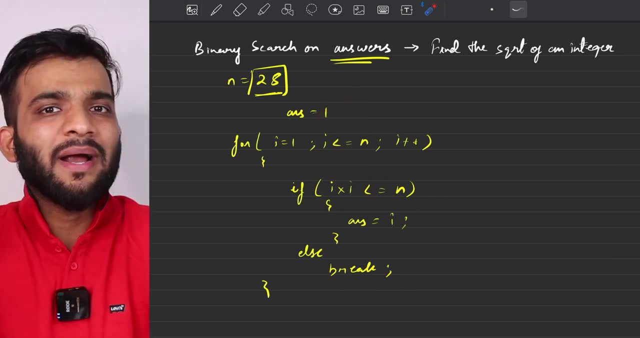 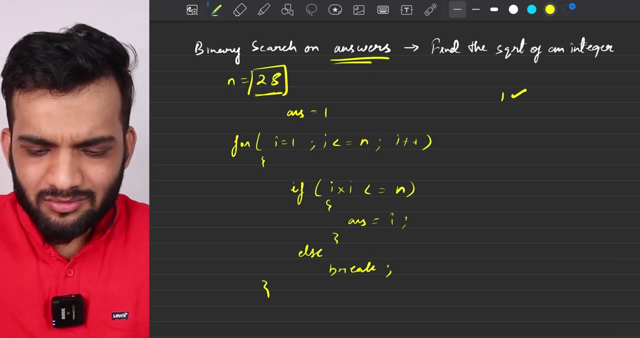 Hence the break statement will be executed and it goes out of the for loop. Essentially, the answer will be stored as 5, and that is our answer. So look at the pattern. Why didn't we stop at 5?? I'm saying 1 might be an answer. I'm not sure 2 might be an answer. 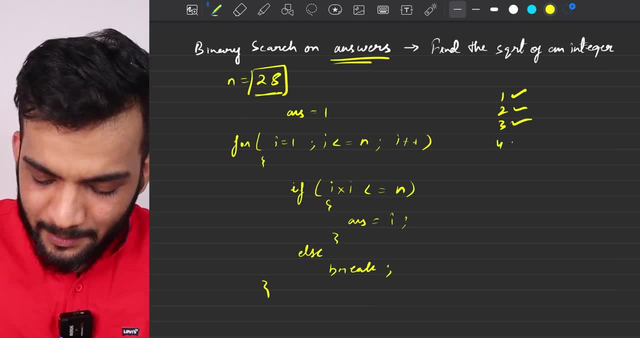 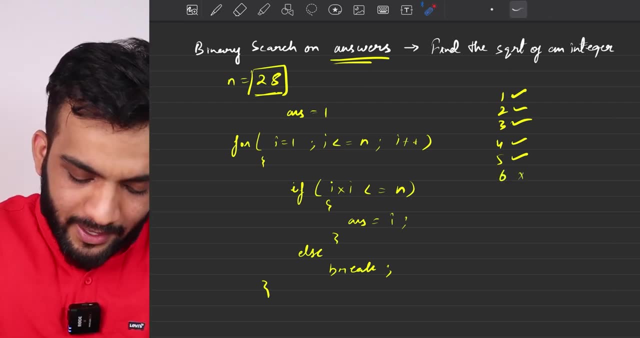 I'm not sure 3 might be an answer. I'm not sure 4 might be an answer. I'm not sure 5 might be an answer. I'm not sure 6 is not an answer. 6 is definitely not an answer. Why? Because 6 into 6. 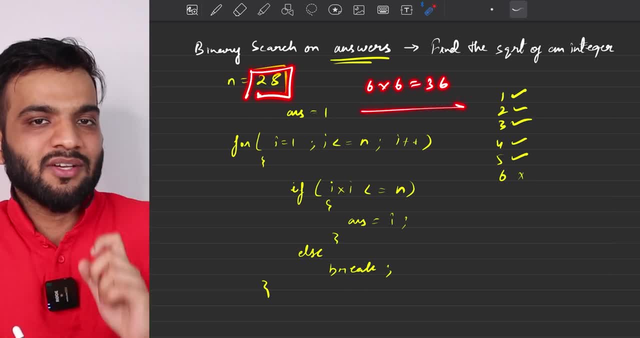 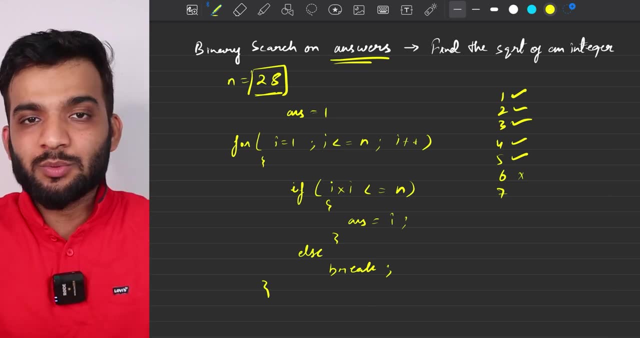 is 36.. And the possible, like the value that is given to us, is 28.. So 6 is definitely not going to be an answer, And I'm very much sure that anything greater than 6, which is 7,, 8,, 9, will never be an answer, Will never be an answer. 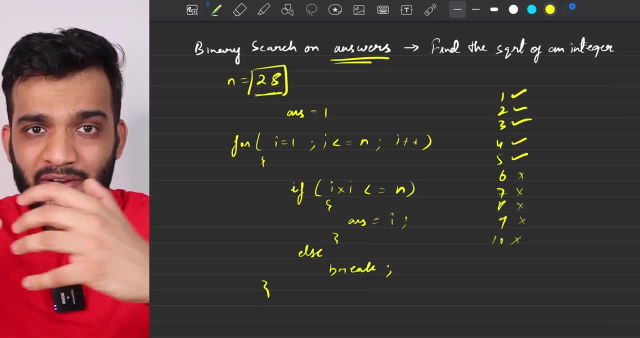 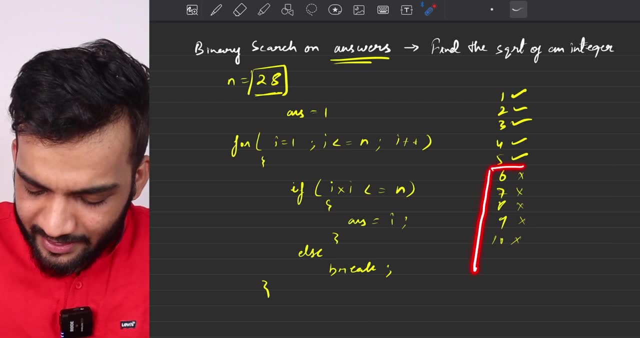 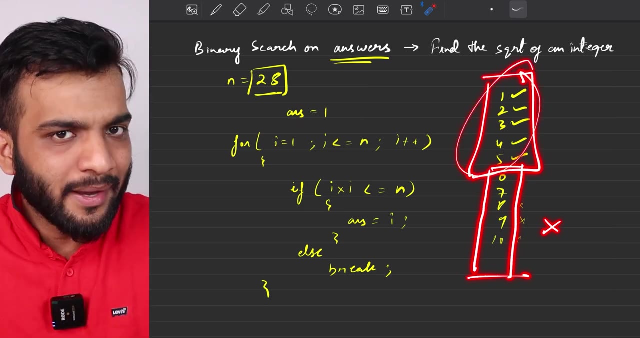 because if you take 6, it's already exceeding. If I take anything greater than 6, that will also exceed Very much. sure Thereby I surely know, anything after 6 will never be an answer, Whereas all of these can be my answer. 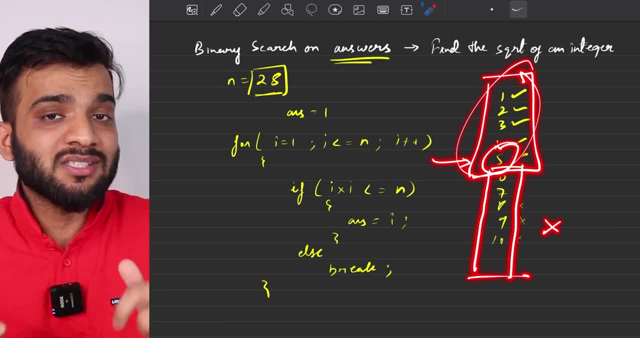 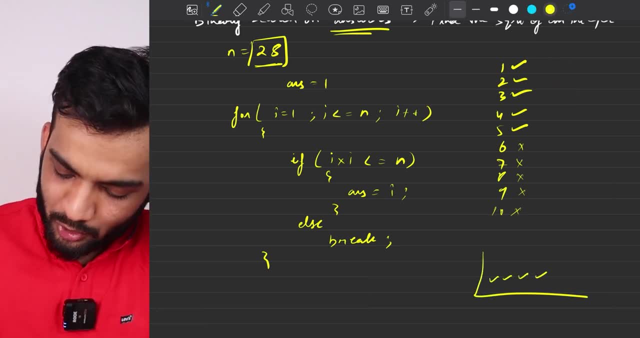 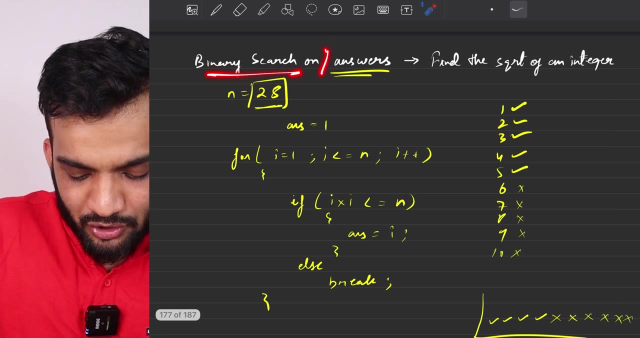 And I take always the maximum value. I take always the maximum value. So whenever you see such cases where till a certain point the answers are possible and after a certain point the answer is not possible, we can always apply binary search on that. Remember this, Why You will. 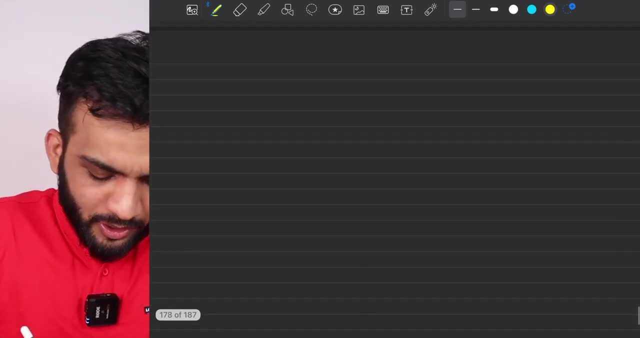 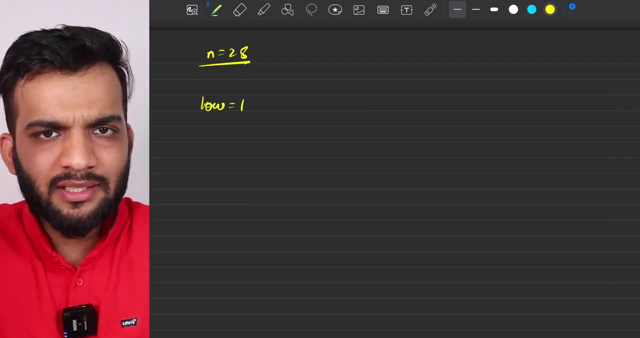 understand as I show you the example. So we're looking for n equal to 28 square root. Can I keep the low as 1?? Like just hypothetically. I'm not doing a binary search on an array. I'm trying to find an answer. 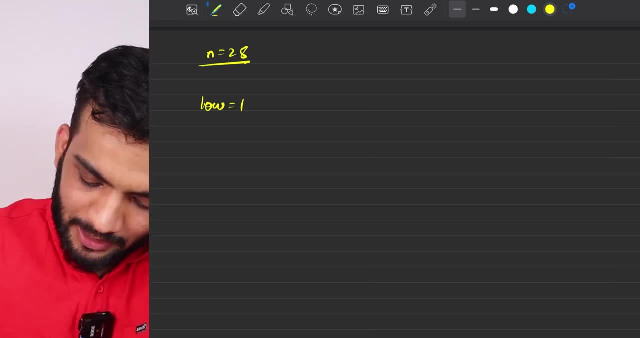 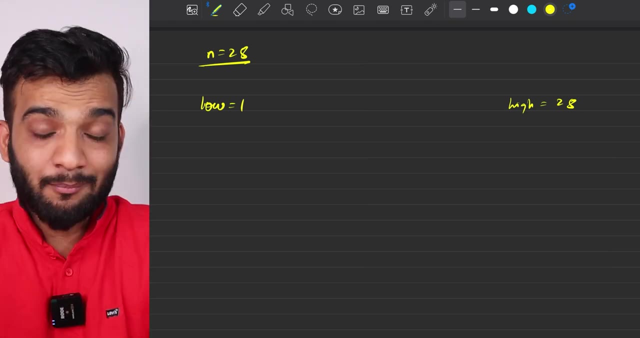 So what can be the minimalistic answer: 1. And what can be the highest answer? That's definitely 28.. Nothing bigger than 28 can be my answer, Like I'm not doing 28 into 28.. I'm just thinking out of the. 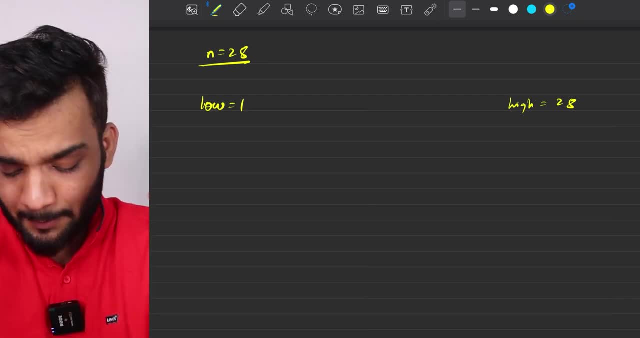 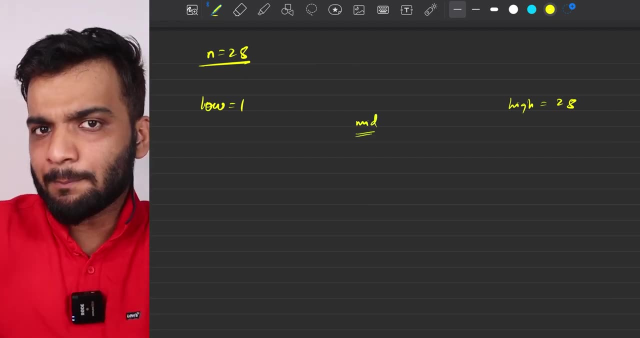 box. Nothing bigger than 28 can be my answer for sure. So I'm keeping low as 1 and we are keeping high as 28.. So if I go across and take the mid value, what would be the mid value 1 plus 28.. 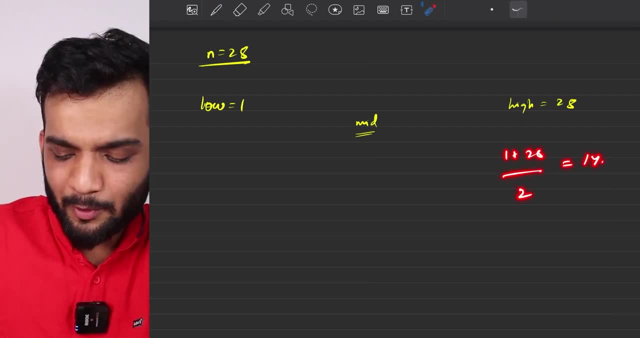 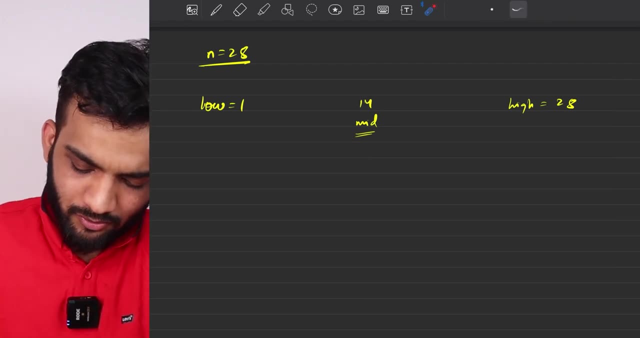 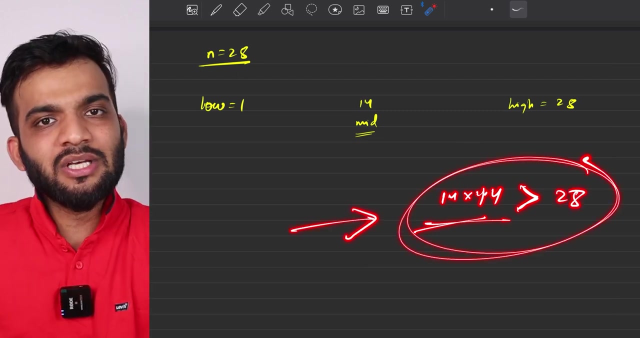 That's 28.. 29 by 2 that's 14.5, that's 14 in integer. so i can write 14. now, if i have to check, 14 into 14 is actually greater than 28. 14 into 14 is actually greater than 28. so thereby can i say: 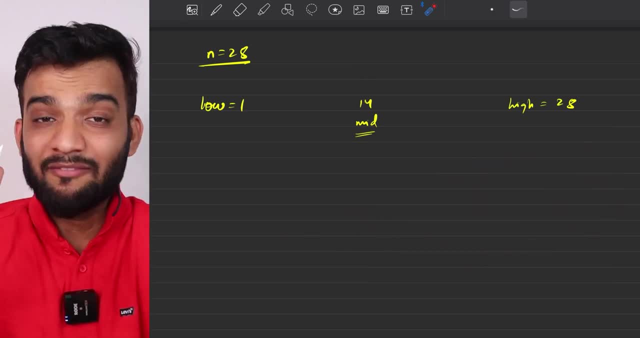 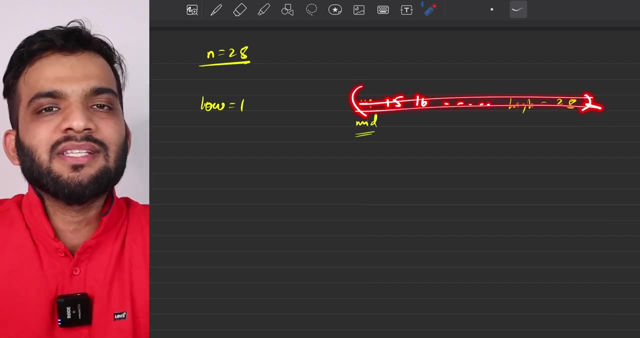 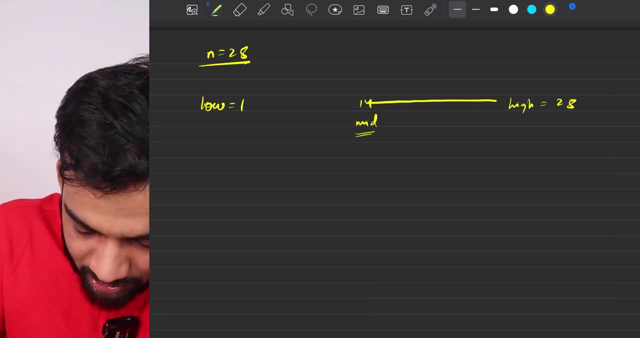 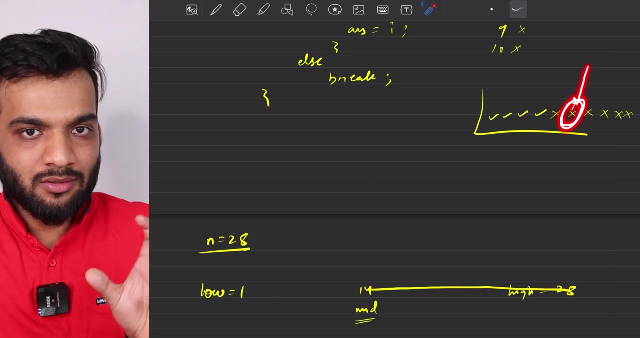 if 14 is not my answer, and i'm very much sure 15, 16 and everything till 28 will never be my answer, can i surely say this? i can, i can surely say this. thereby, what i do is i eliminate everything on the right. why? just because of this reason, if i'm standing at a not possible stuff, everything. 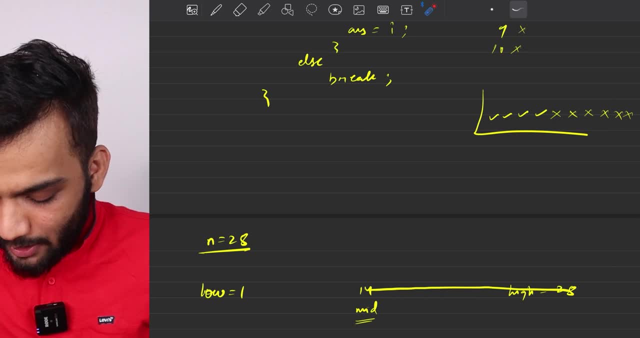 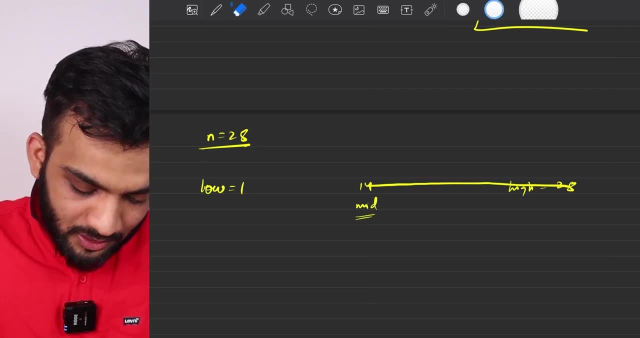 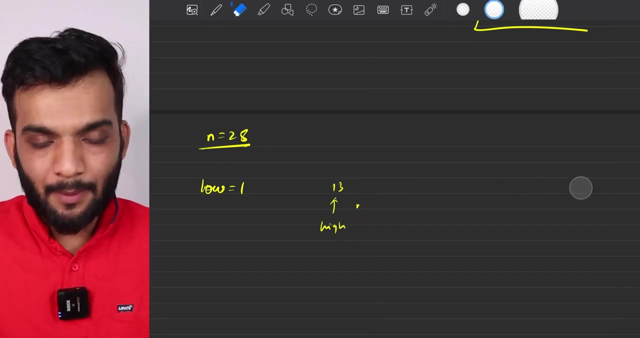 on the right will also be not possible. so why do i consider the right portion? so what i do is i eliminate the right portion and the moment i eliminate, the high will be coming across to 13- 13, the high will be coming across to 13. so we're just playing around with numbers, not taking any array. 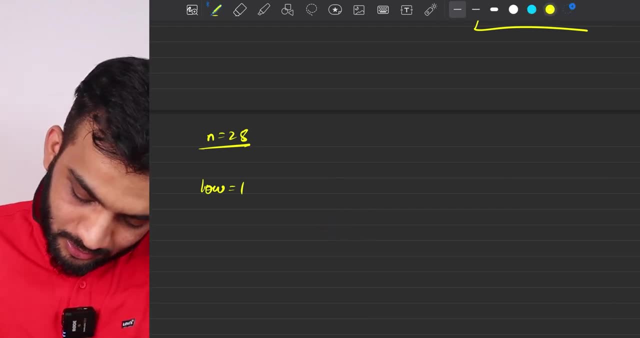 so high is 13. let me write that. so the high is 13 this time. where will the mid point to? can i say the mid will point to 13 plus 1, that is 14 by 2, 7 obviously will 7 be. my answer: 7 into 7 is actually. 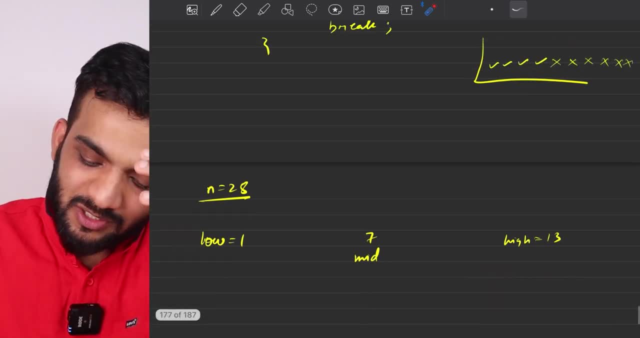 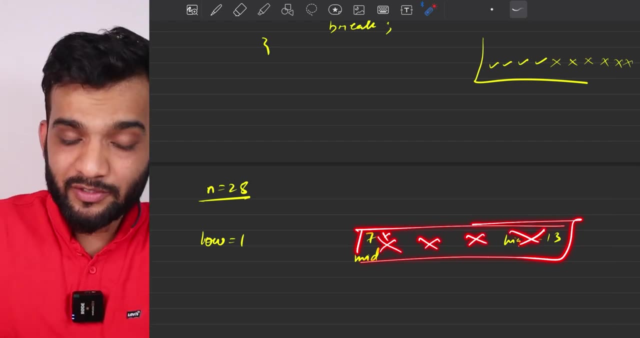 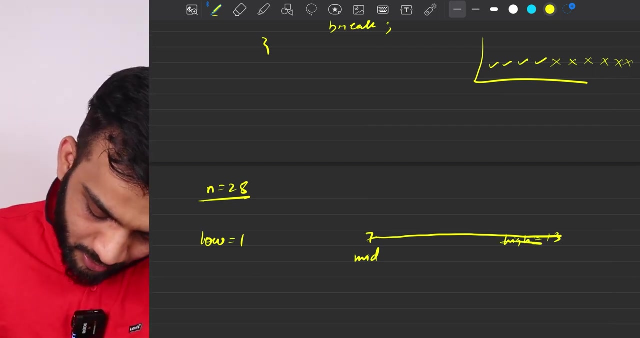 greater than 28. so 7 also cannot be my answer. again, i'm standing at a not possible. so can i say everything? so the right of 7 is also not possible, obviously no. thereby i say everything can be cancelled. hence this high will move to 6, which is one place before mid. simple binary search. 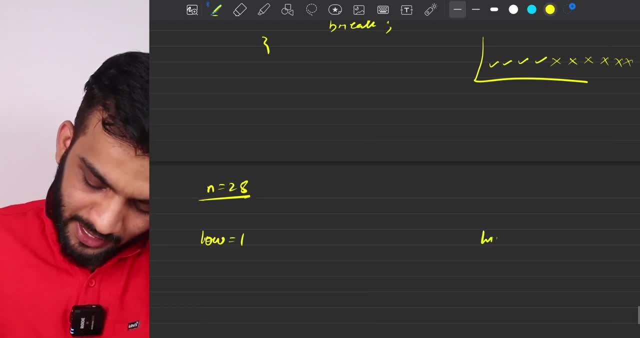 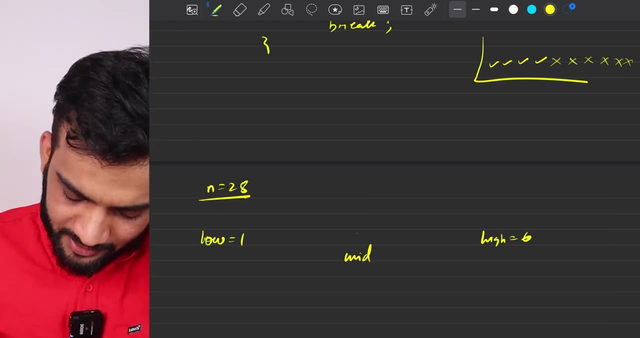 eliminating the right half, high will be 6. perfect. what will the mid this time? 1 plus 6 is 7, 7 by 2 is 3.5, so thereby the mid will be 3. this time 3 into 3 is not possible. so i'm standing at a not possible. 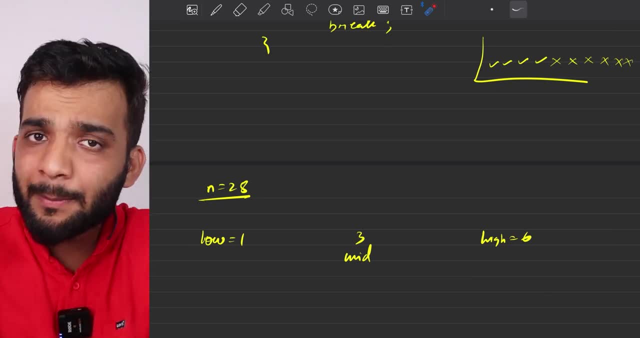 so the right of 7 is also not possible. so i'm standing at a not possible. so i'm standing at a not possible greater than 28. so i'm saying, maybe this 3 is an answer. why? because 3 into 3 is lesser than equal. 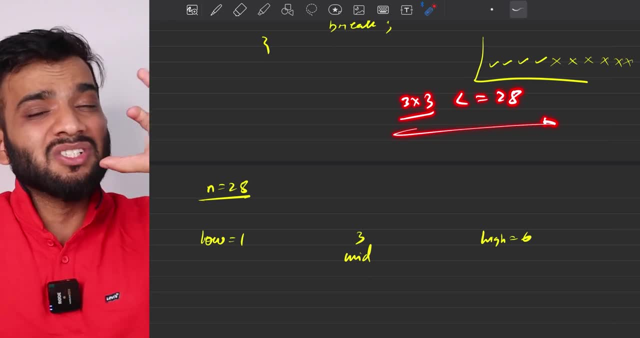 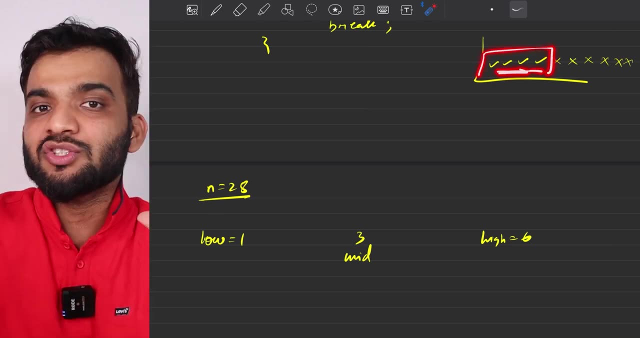 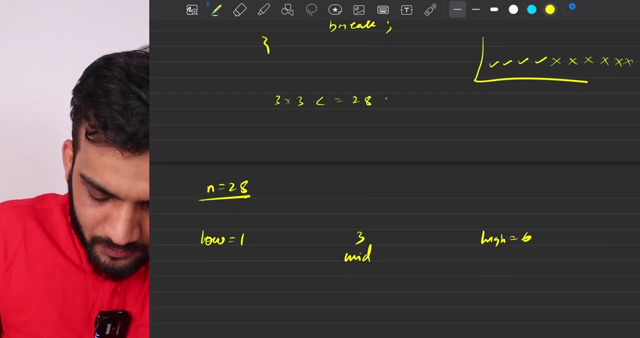 to 28. i'm not sure that this is an answer or not, but this might be my answer. like, probably i'm standing somewhere here, so this i'm standing in this possible section. probably 3 might be my answer. why? because 3 into 3 is lesser than 28, so it's not this square root, but it. 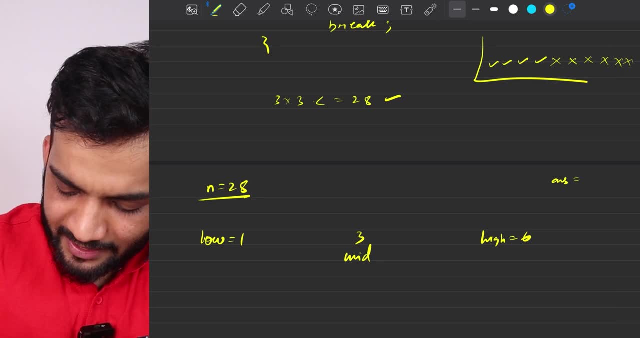 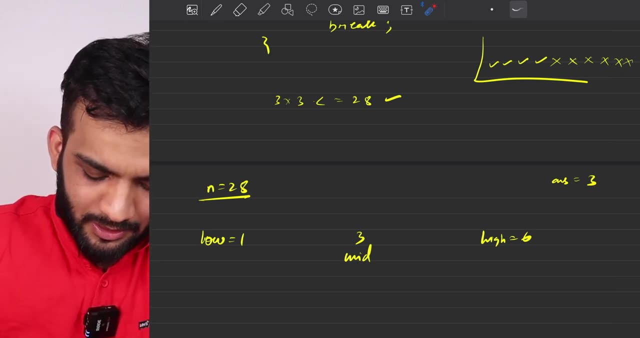 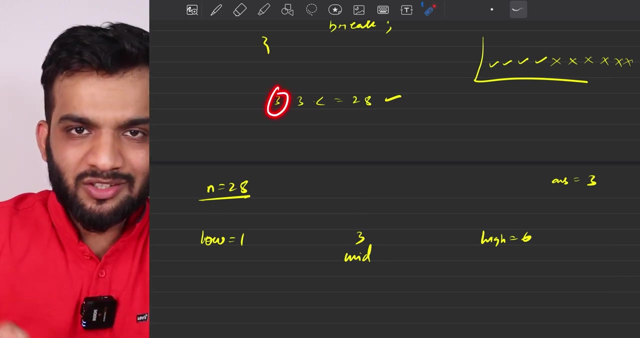 might be my answer. so I'm saying: hey answer: can you store three? hey answer, can you store three. he says, okay, let me store three. now tell me one thing: if I go on the left, will that make sense? or shall I go on the right to find a bigger number? because if I've got three, obviously two. 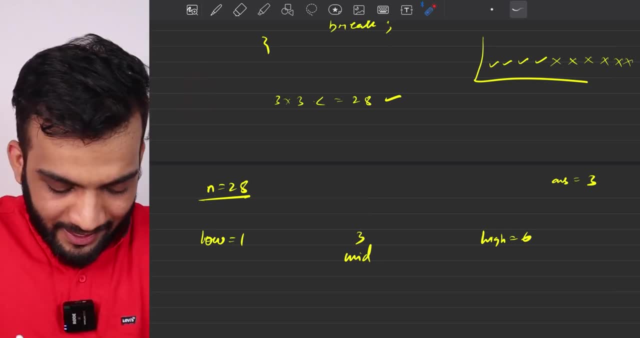 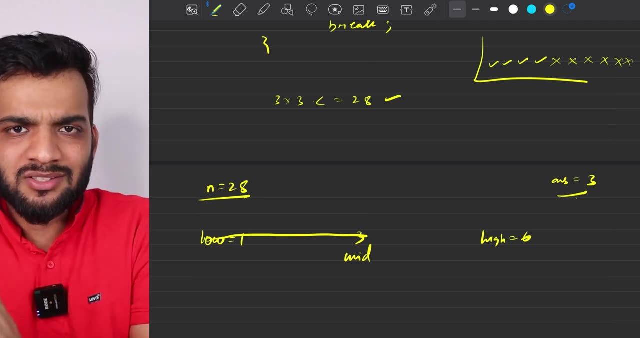 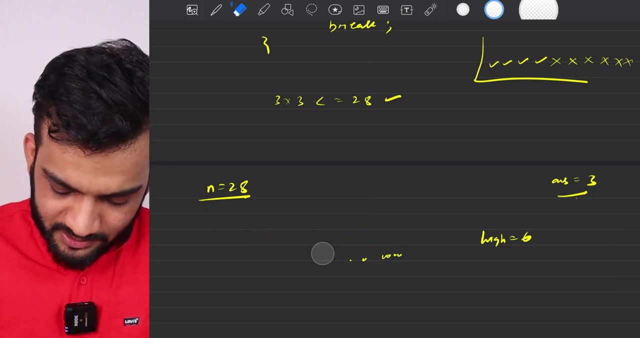 will never be my answer. obviously, one will never be my answer. so can I surely say: anything on the left will never be my answer. I have taken the assumption of three being my answer, but anything on the left will never be my answer I can. thereby the low will go to four. perfect, let's take the 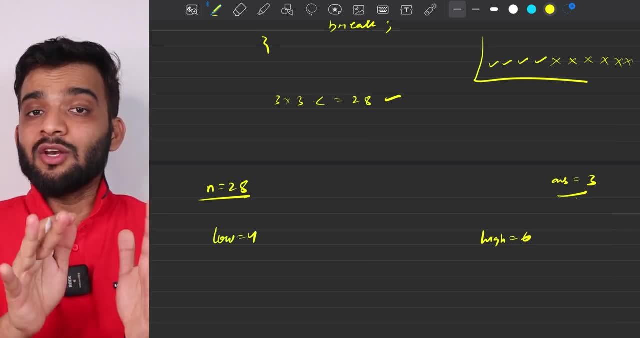 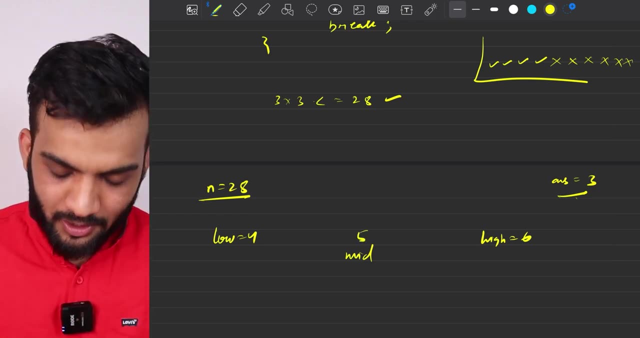 low to four. so the moment I take the low to four, this time the mid will be low plus five. four plus that's 10, 10 by 2 is 5. so I have 5. the moment I have 5, what do I check? I again check the same. 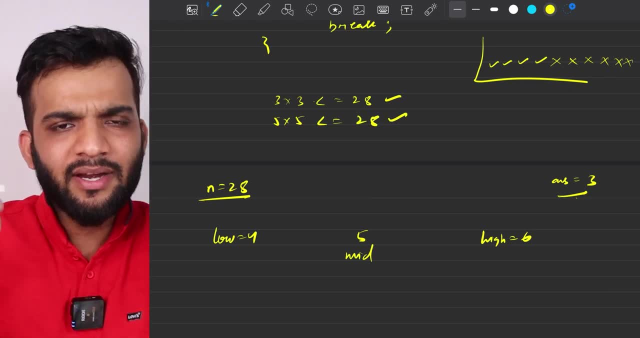 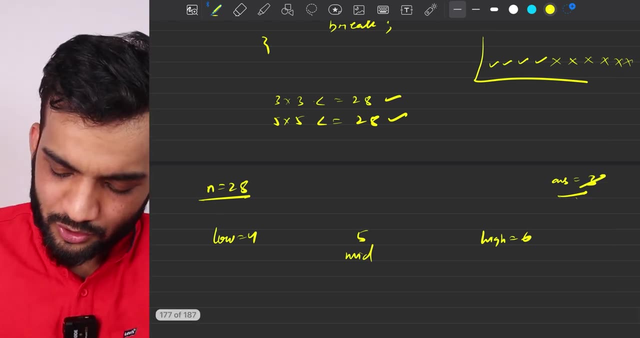 thing, 5 into 5, lesser than equal to 5 to 28, and i find, yes, it is, 5 into 5 is lesser than 28. i say, answer, you got someone better. please replace yourself, because i'm looking for square root and i'm going to the right to find the. 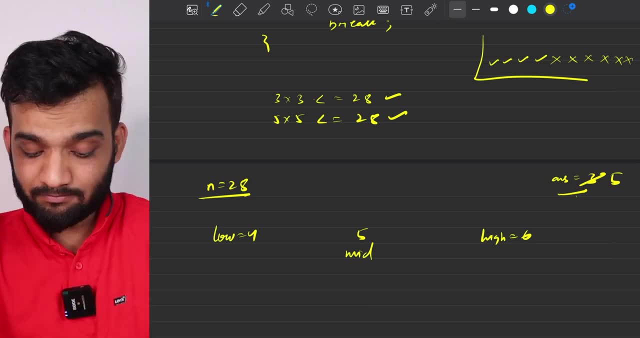 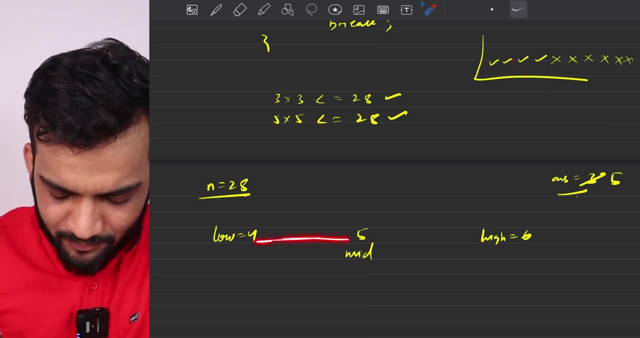 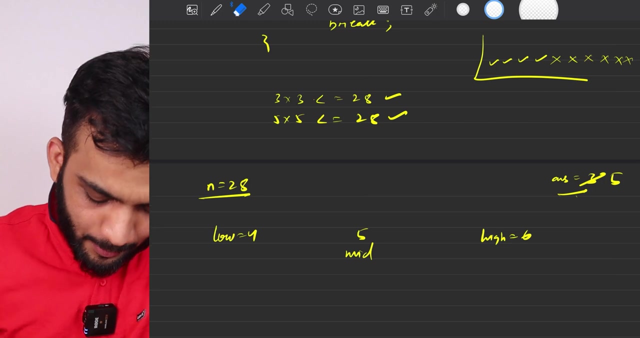 biggest value that is less than equal to 28, i've got 5. so i know one thing: probably i'm standing somewhere here and i can surely say anything to the left. i don't need it. i need the biggest value that is close to that value. when i do a multiplication thereby, i say: can you please? 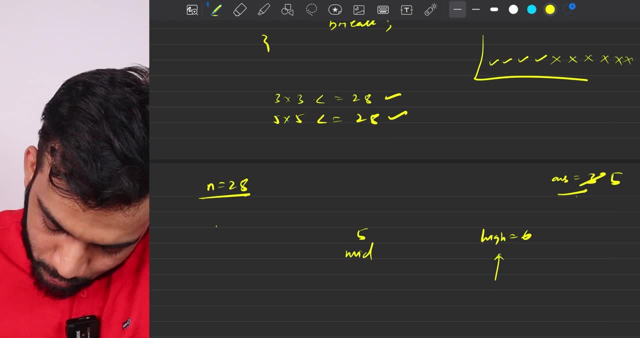 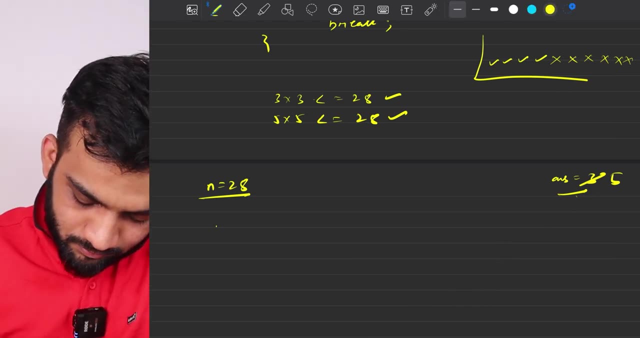 eliminate and take the low to this portion, which is one place ahead of mid that is at high. thereby we are at six and the low points here and the high points here and the mid also points here. so currently we're standing here, point to note, we're standing at a single value and 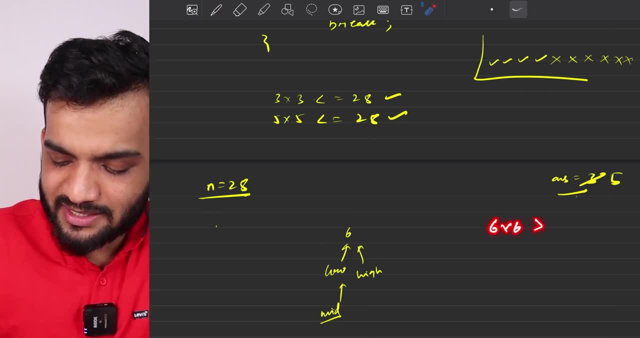 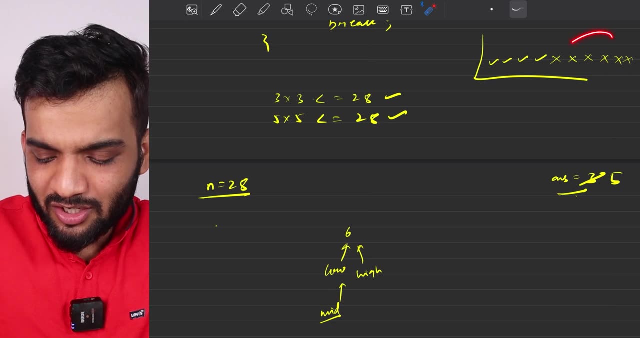 this time i do 6 into 6. that's greater than 28, so 6 cannot be my answer, 6 cannot be my answer, and if it cannot be my answer i say i'm standing under this portion. thereby the right portion will be eliminated, and 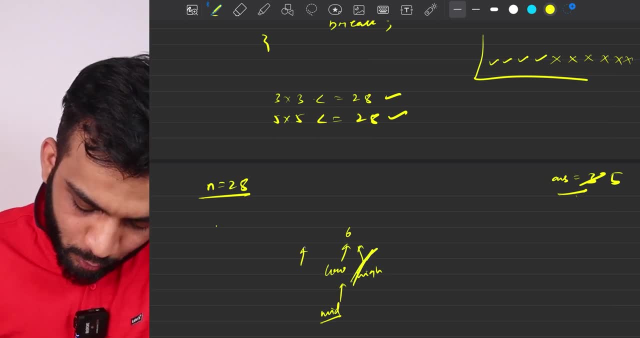 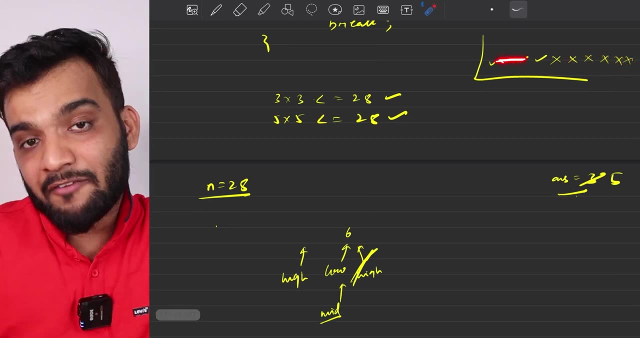 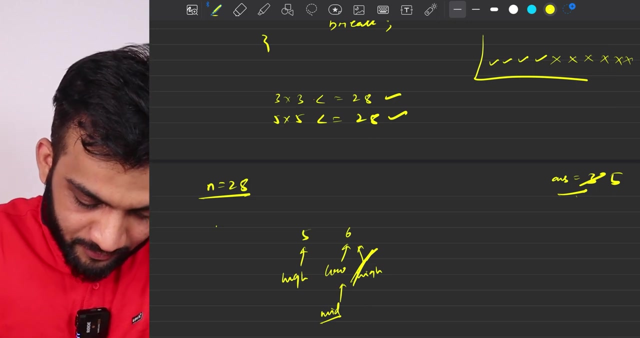 if the right portion is eliminated, the high will always move one step back. if the right portion- remember this- if not possible, the right portion is eliminated. if possible, the left portion will be eliminated, because i'm looking for the possible answers. thereby, what happens? i take the high to 5. 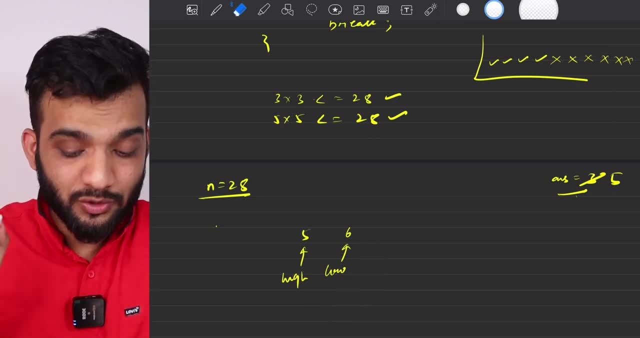 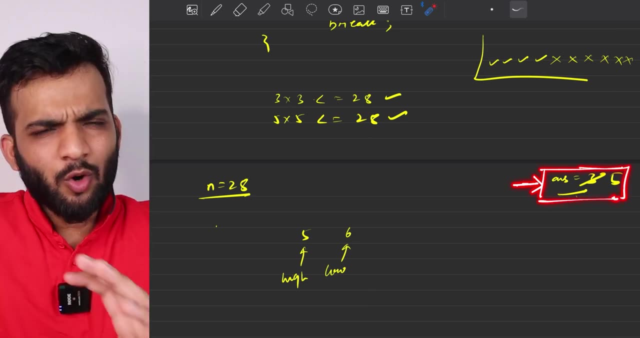 and this is where we end. this is where the binary search will end. so, if you remember, in the initial lectures i told you one thing: as of now, you can play with this answer and you can always store your binary search answer. but eventually, as you go through, you'll understand that one of the high 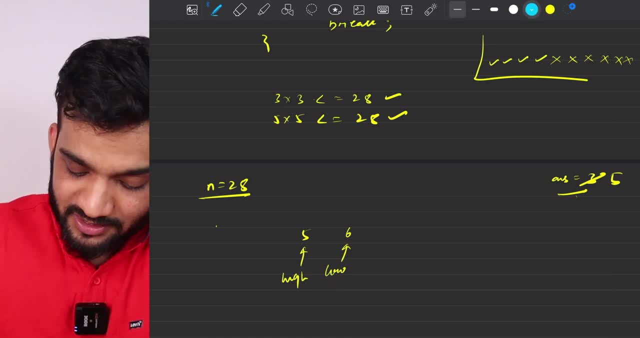 or one of the low will always be pointing to the answer. so in this case you can see that this variable high is actually pointing to the right and the low potential answer. you can notice that the keep delay is always pointing to the left and the upper funet is pointing to the right, and 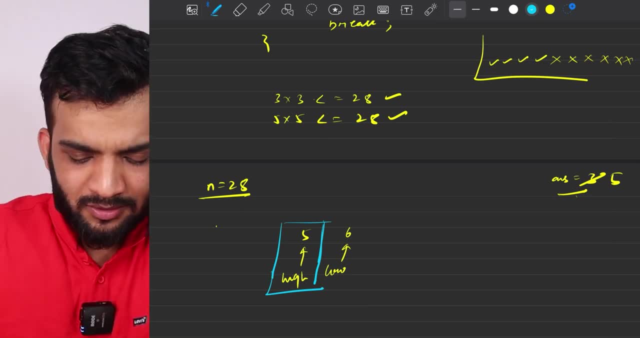 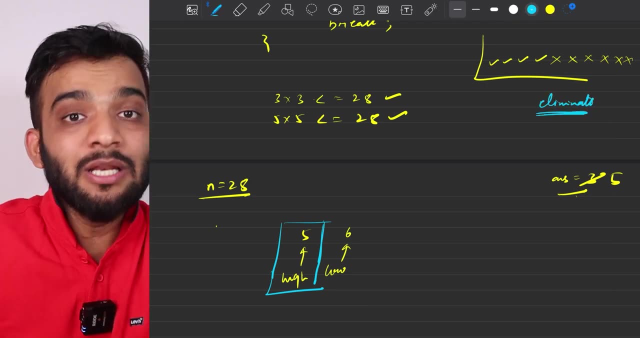 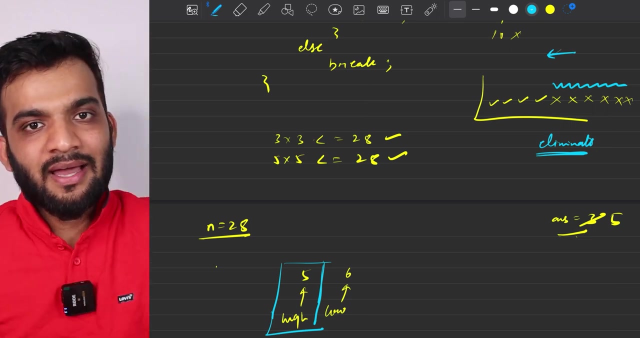 to your answer, that is five. and why did that happen? the sole reason is: since you're trying to- i'll just write it for you- since you're trying to eliminate, since you're trying to eliminate, and this is the not possible zone, so you're trying to move on this direction and that's why the high 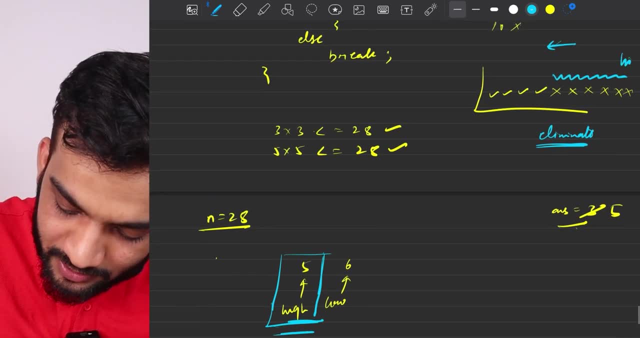 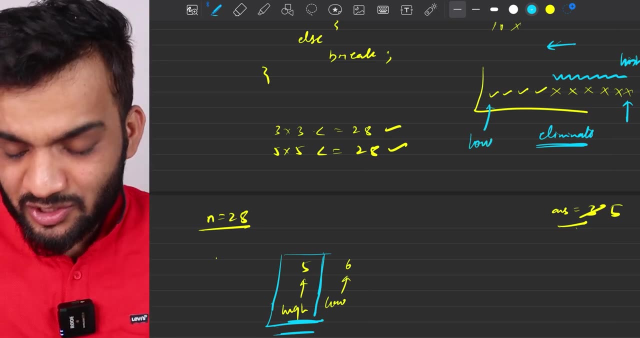 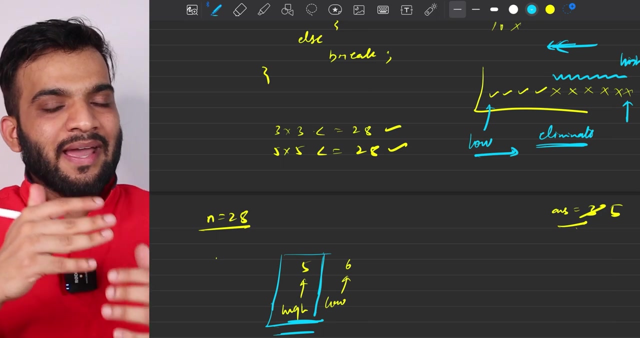 will cross the low and when you're trying, because high was here initially at a not possible place and the low was at a possible place. so, since you're eliminating thereby, the low will always move towards right and the high will always move towards left, hence the low ends up pointing the 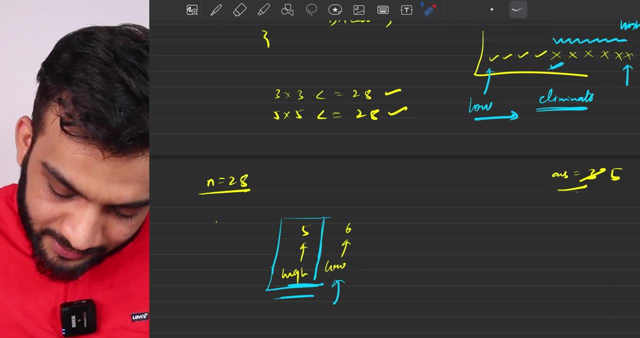 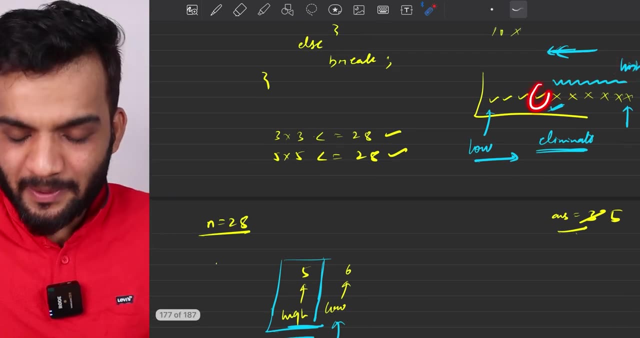 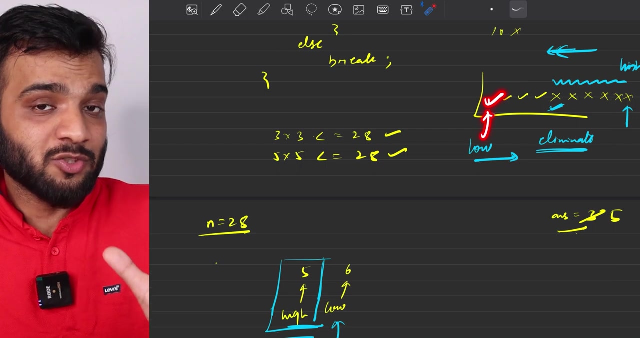 low ends up pointing at the first place, at the first place where it is not possible, and the high and the high ends up pointing at the first place which is possible. so, to repeat, the low was, at at A starting, pointing to a place where it is possible. the high was pointing to a place 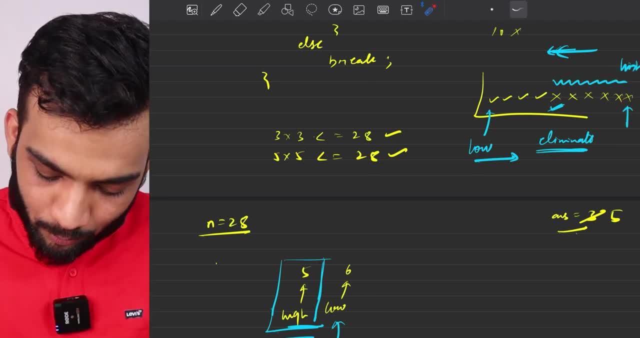 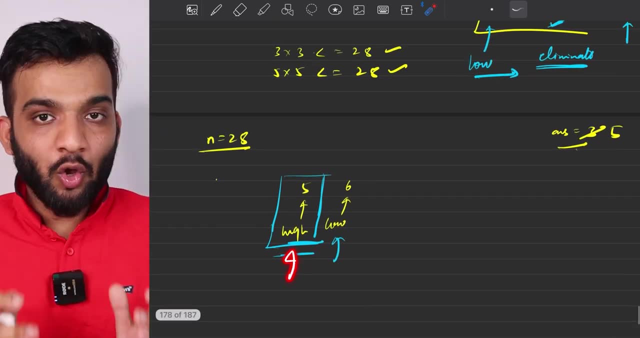 where it was not possible. they're trying to move and, on moving, they'll come to a place where it is not possible. this will come to a place where it is possible. hence, the high will always be storing your answer. so, in order to understand this much better, what i'll tell you is: take some more. 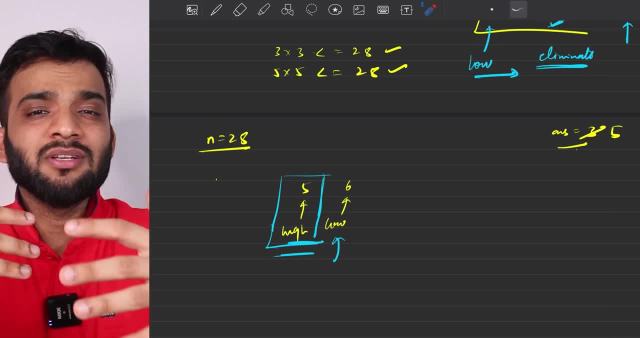 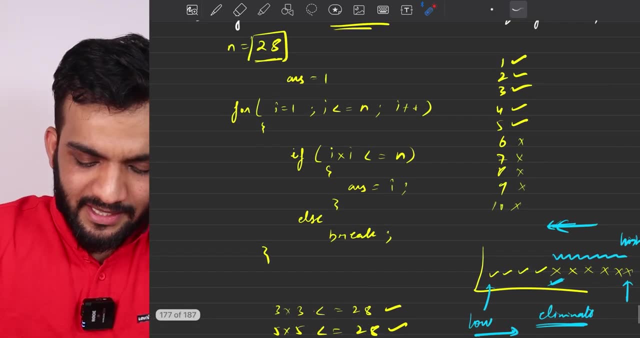 examples and take your pen and paper and try to do the dryden and you'll eventually understand how does the binary search work in this case. so we have pretty much done this stuff. can i say that this line was the linear search and because of this line, the complexity. 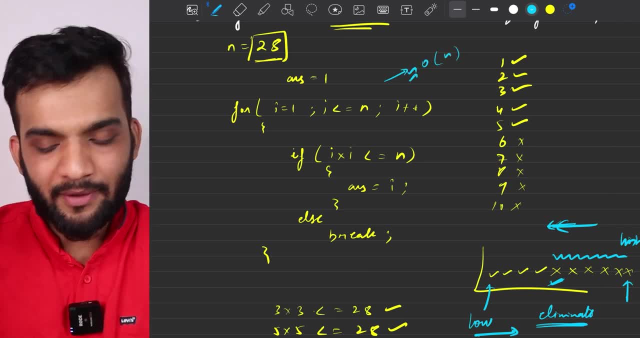 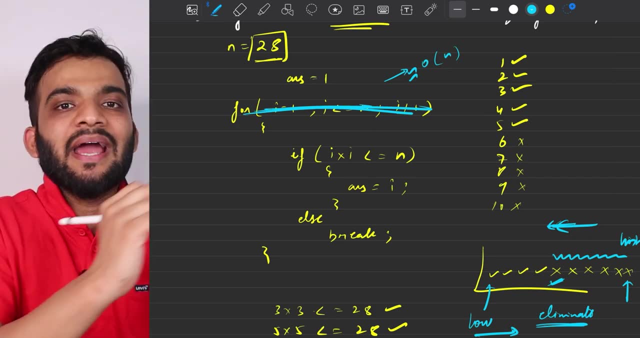 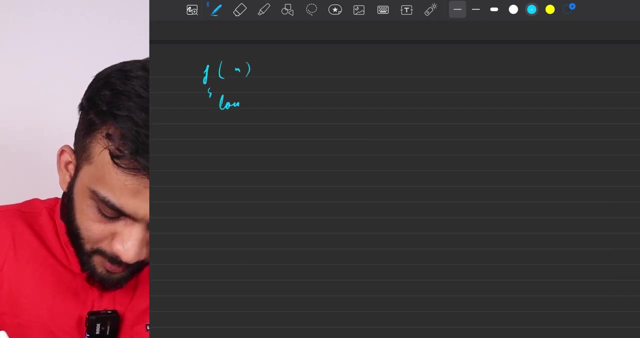 was near about bigo often, near about bigo often. but. but this concept will now be replaced with binary search because i'm not going through the iterative stuff. instead of that, what i'm doing is i'm saying: hey, listen, you're given a number. thereby, the low will be one, the high will be. 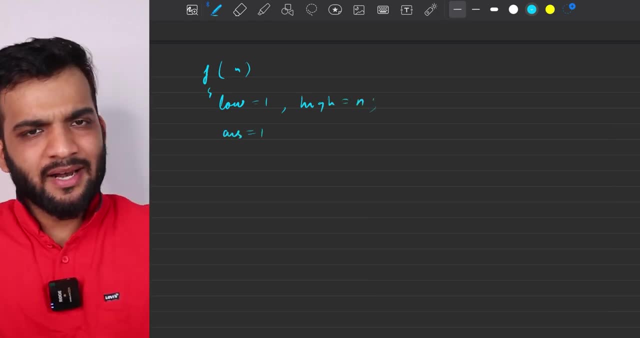 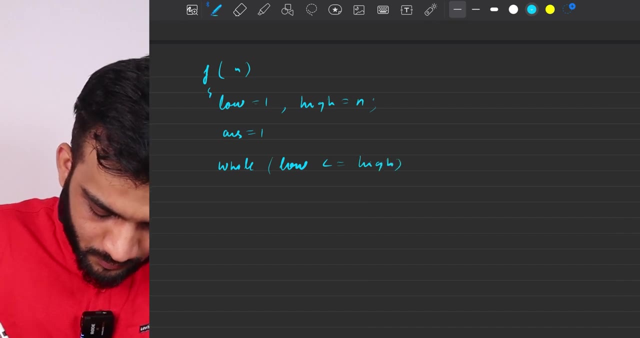 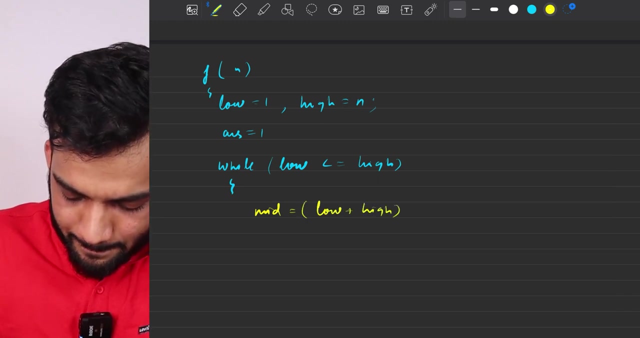 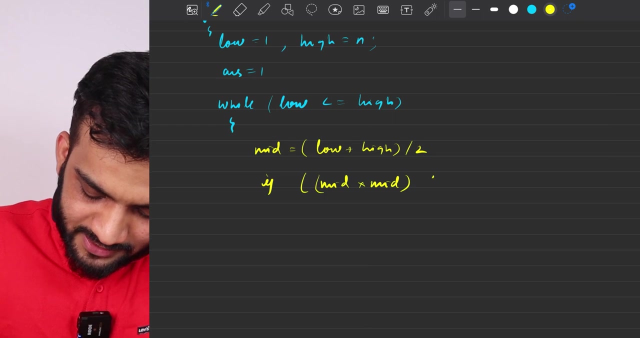 n in this case, and we can keep the answer so that you can understand it in a much better way. i can say: while low lesser than equal to high, and inside that i can write mid equal to low plus high by two, and after that can you say: if mid cross mid is lesser than equal to the n, then your possible. 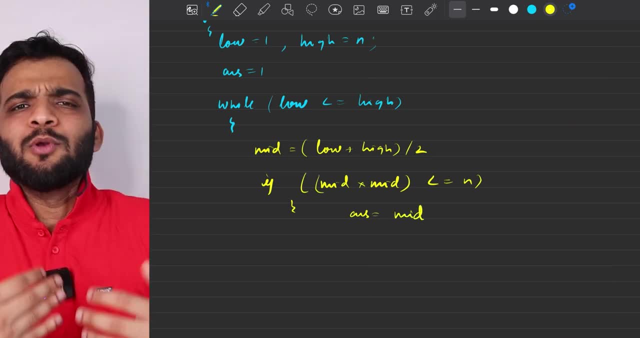 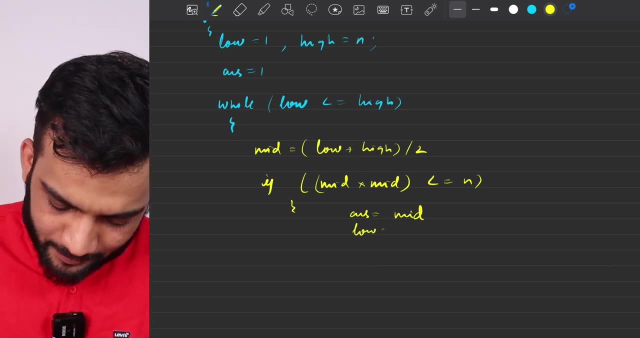 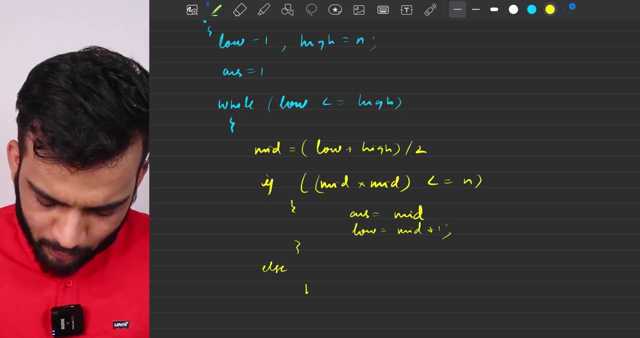 answer can be this: mid can be, but i'm looking for a bigger value every time because this might be it, but maybe someone else can be. so i will always go and eliminate the left half and i'll move on the right- perfect. or else, if this is not possible, this is not an answer- look for smaller. 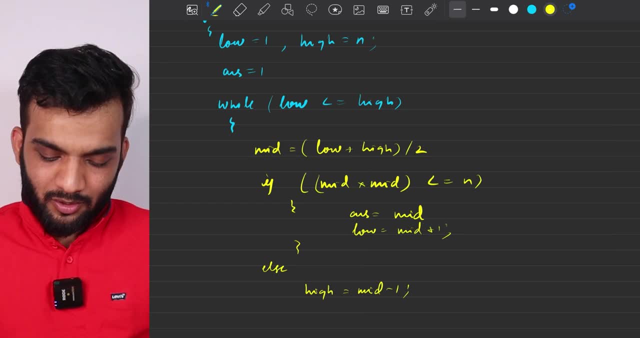 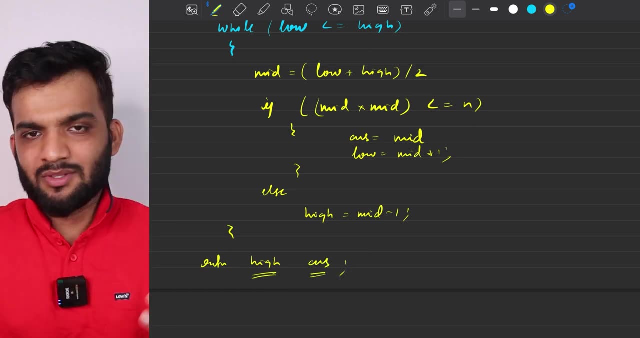 values, look for smaller values. that is, eliminate the right half. quite simple. once you're done with this, either you can return the high or you can return the answer. that is your choice. you can either of them and that will work. so, if you remember, at the beginning of this lecture i told you that we 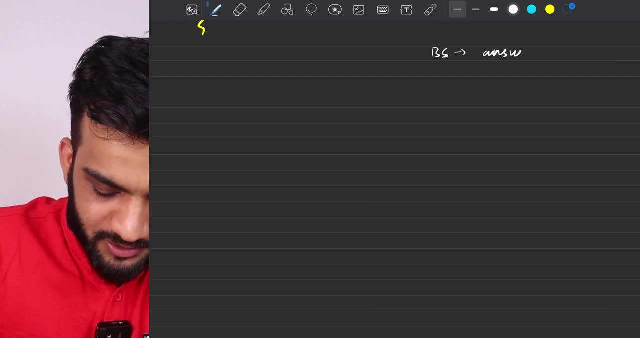 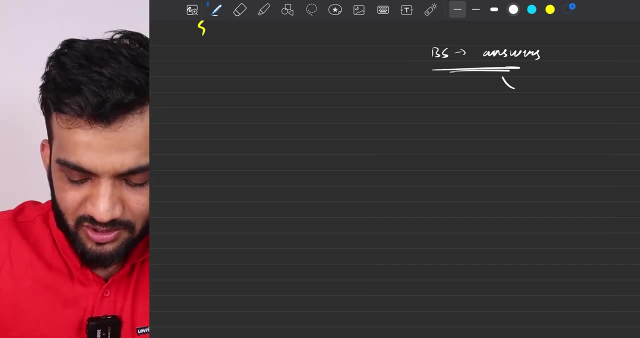 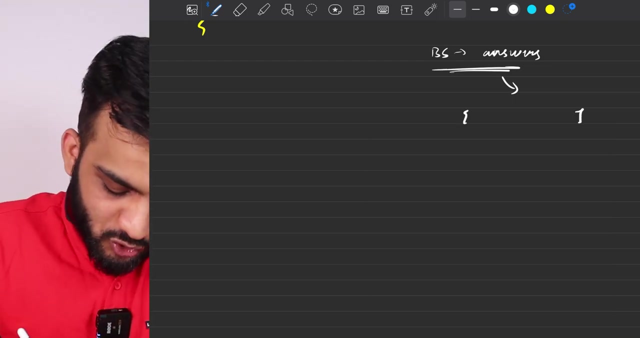 will be doing this pattern: binary search on answers. so remember one thing: whatever problem you will see in the future on binary search on answers, they will always be focused on this thing: that you always know the range of answers. like in this question, i was being asked to find the 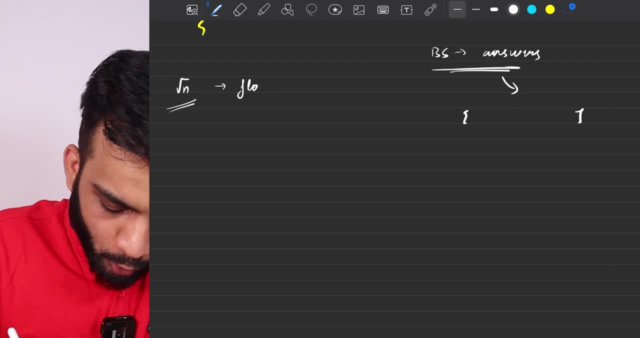 square root of n and it was being asked floor of that square root of n. that was the question. or, if i have to like, modify the problem statement, it will be: find the maximum integer, find the maximum number or integer which, on squaring, is lesser than n. can i say this because 5 was the maximum integer which, on squaring, was lesser than. 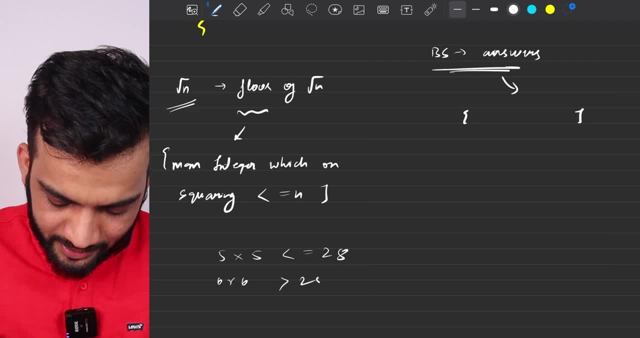 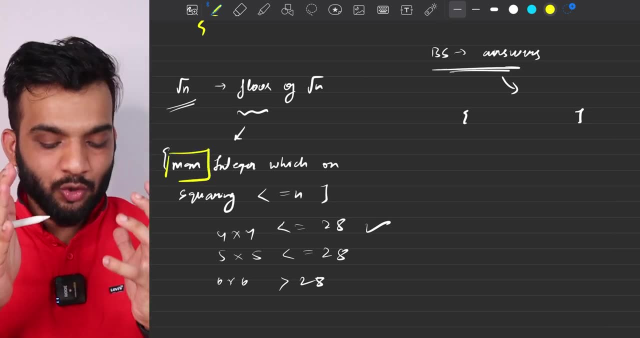 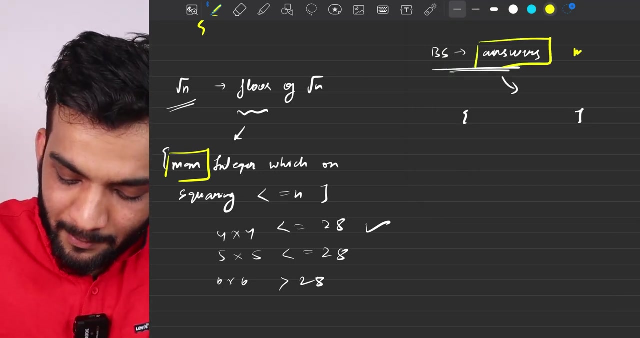 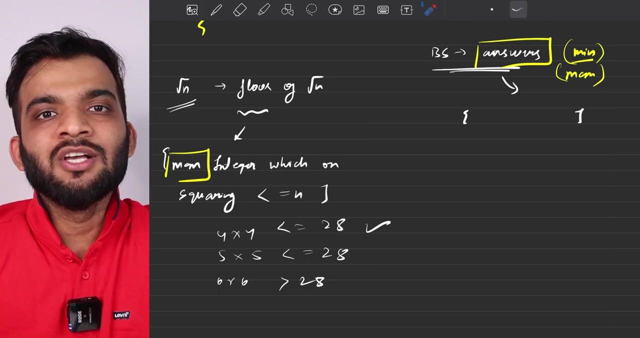 equal to 28 because 6 on squaring was greater than 28. 2018. that was also possible as well, but i was being asked to figure out the max integer. so, across all the questions on a this area on answers, it will be asked to find. 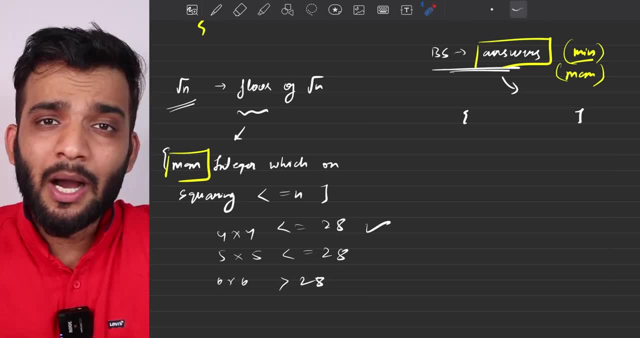 minimum possible integer or maximum possible integer, which can be your answer. problem statements will vary and we're solving a bunchi are those in the upcoming lectures, but remember, whenever you see min or max, find out the minimum possible integer, called max, and the problem statement on the walki see every but i students learning which answer plus some questions and 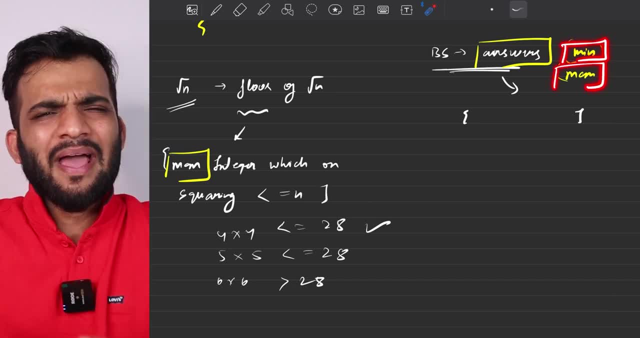 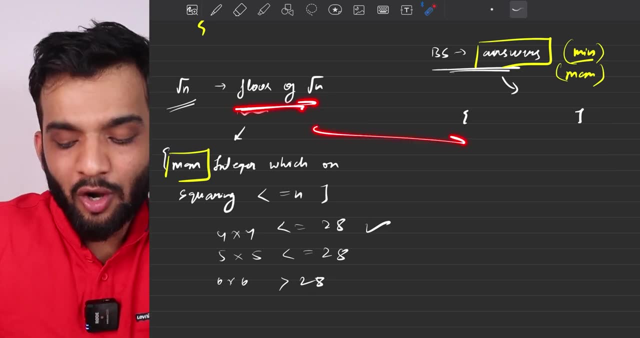 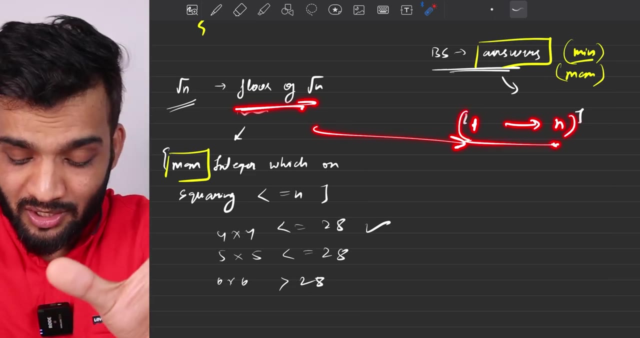 but remember, whenever you see something like min or max, find out the minimum integer. find out the maximum integer. and and if in a question you're sure that the answer- like in this case, the answer was always between one and n, if you're sure about the answer range and they're asking you to find 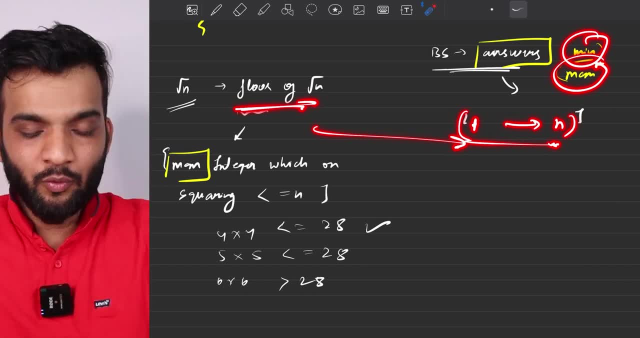 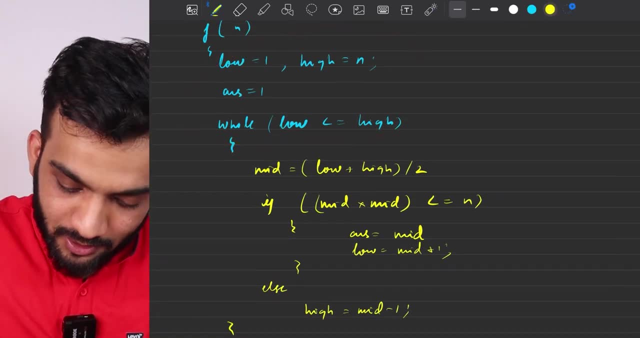 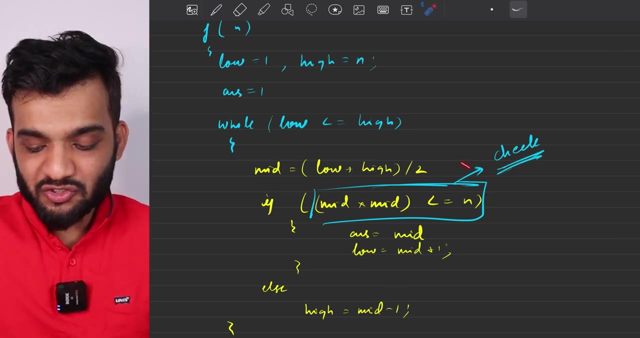 the minimum and maximum in that answer range: always, binary search always. and the pattern will be very simple: you do the binary search and this method, this one, is known as the check box. it is the check, because this was the question, this was the question, check condition. the question was: 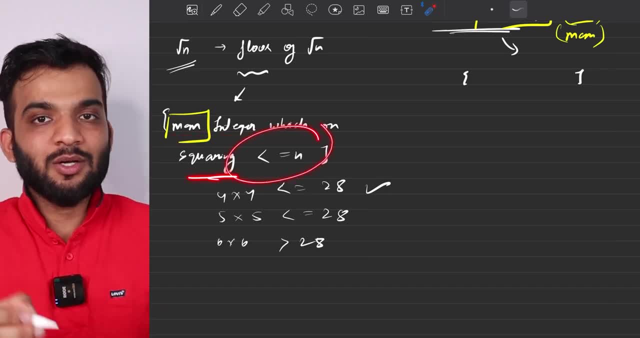 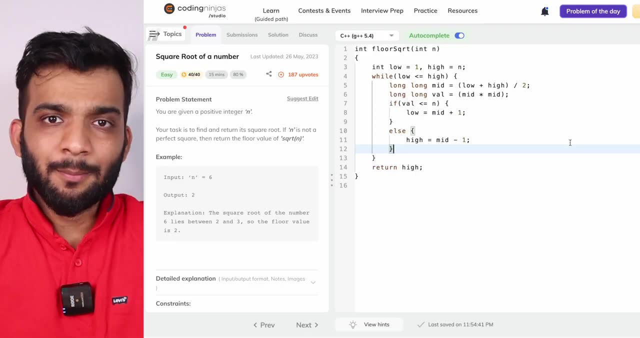 stating maximum integer whose squaring is less than equal to n. and that is what i did. the check condition, binary search under the check condition got it. let's quickly jump into the code editor. by the way, you can find out the problem link in the description. so the first thing to observe is: uh. 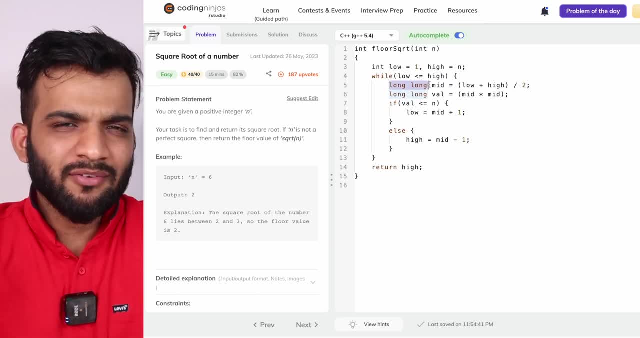 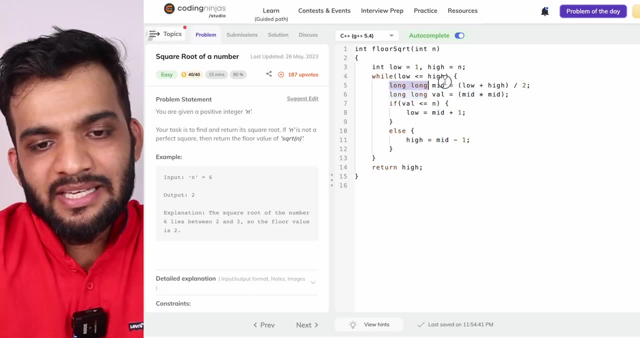 i'm taking long long why? because imagine you've been given 10 to the power 9 as n. so the moment you do 10 to the power 9 into 10 to the power 9, it might overflow. so just take care of that and take long, long. so 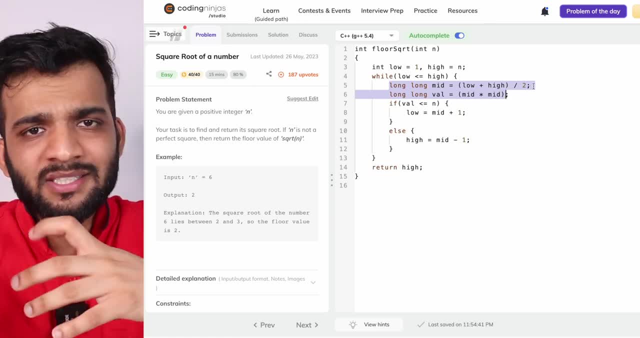 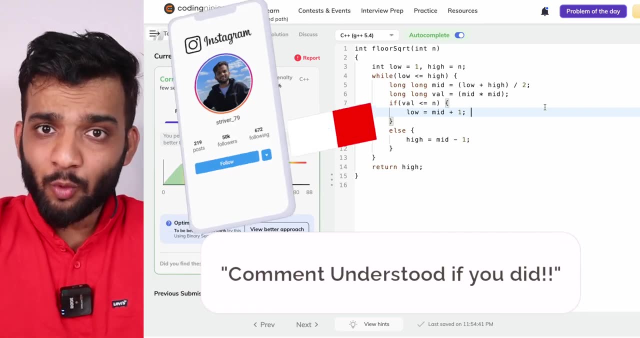 in certain cases. you have to keep this in mind, otherwise there will be overflow cases and you'll get a wrong answer. so if you try to submit this, this will be running absolutely fine. so i hope you have understood everything and in case you're still watching, please, please, do consider giving us